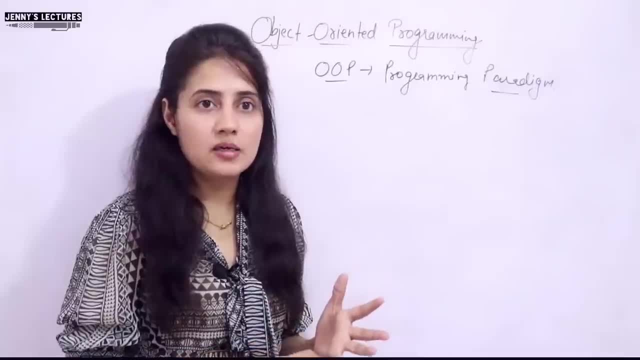 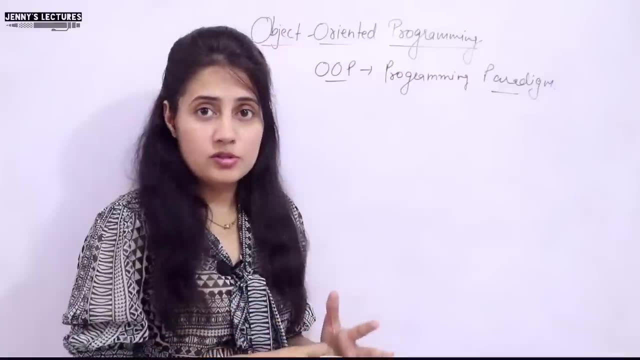 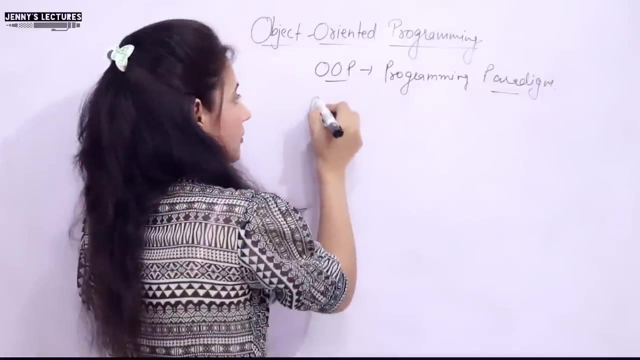 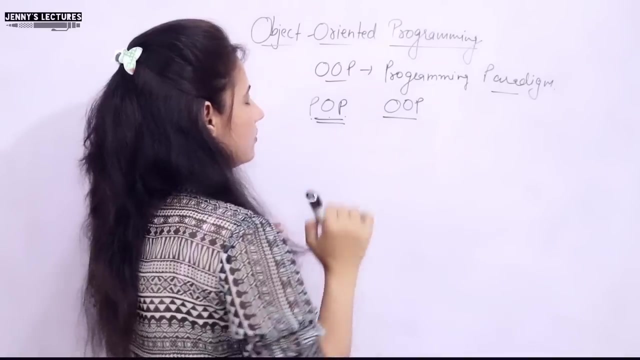 right, imperative, functional, parallel. under imperative two types of paradigm comes, like procedure oriented and object oriented right. So different, different paradigms are there. Basically, main are procedure oriented paradigm, procedure oriented programming and object oriented programming. these two right, These two comes under imperative, imperative programming. 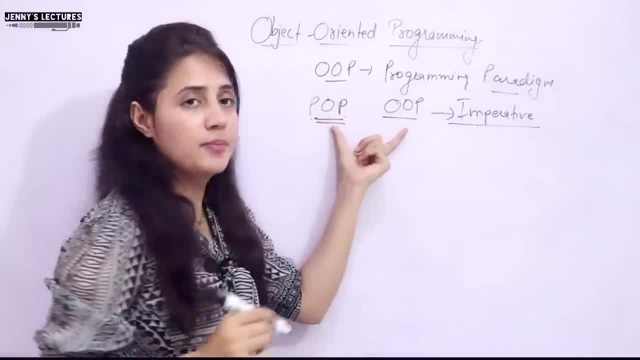 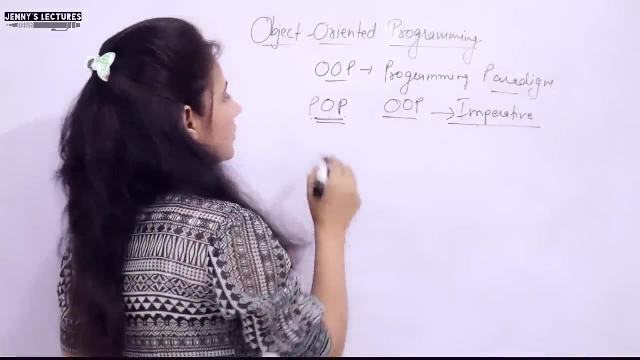 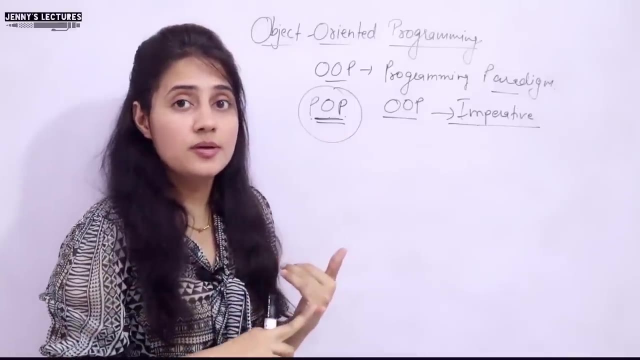 paradigm. these two comes under this category: imperative programming paradigm, POP and OOP, in which we more focus on how to do the task rather than what to do right Now. what is this? procedure oriented programming, As the name suggests, procedure oriented means. procedure means how to do a particular task, right the steps or, in this, this computer or programming. 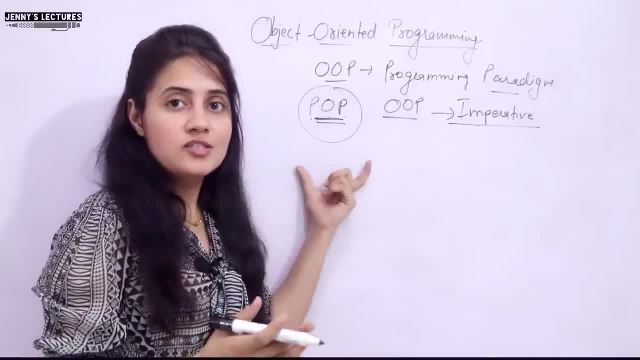 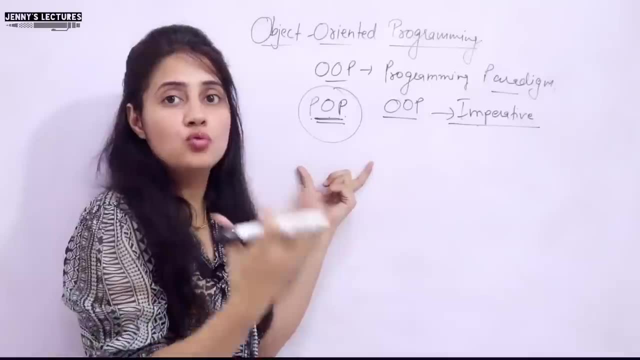 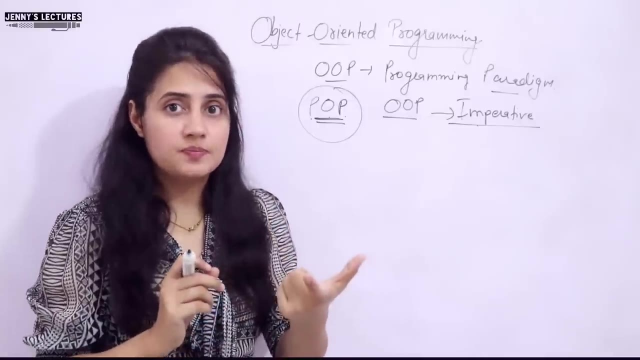 language terms we can call that algorithm, So this would be oriented. this would revolve around the procedure, right, Main focus is on the algorithm: how to do the task rather than what to do. fine, and procedure. we can say procedure or function- right same thing. 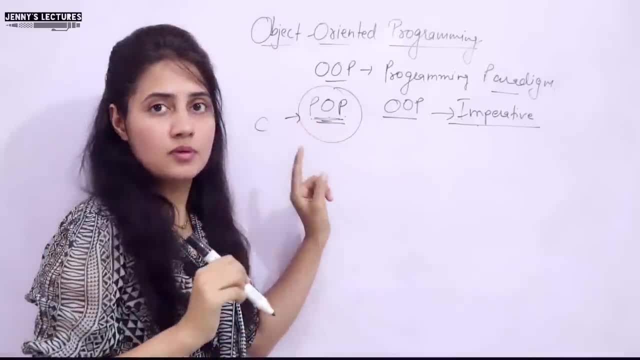 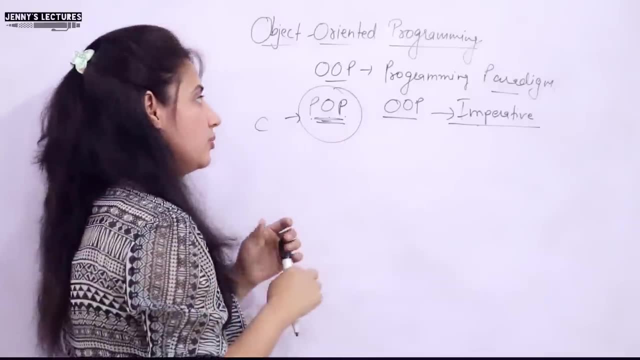 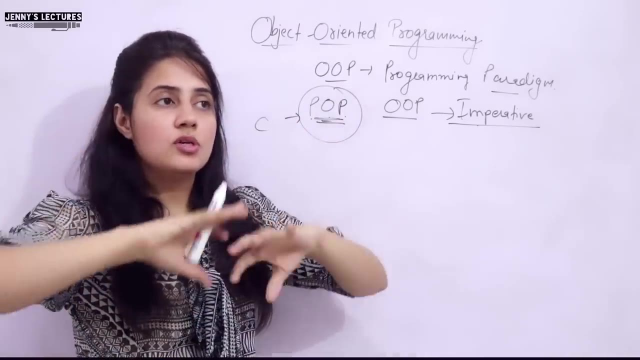 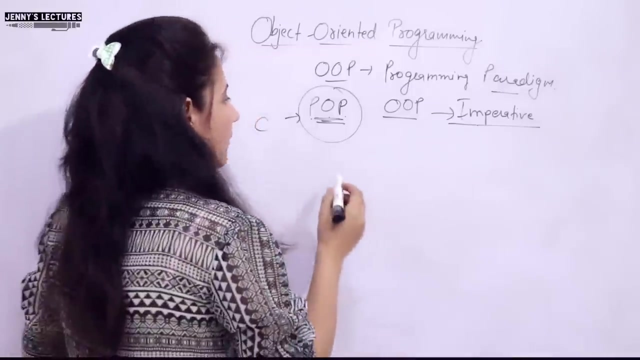 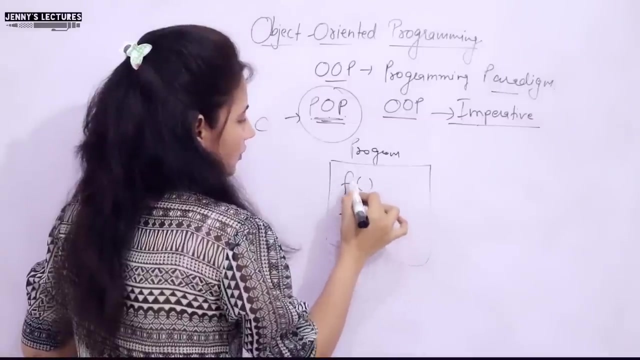 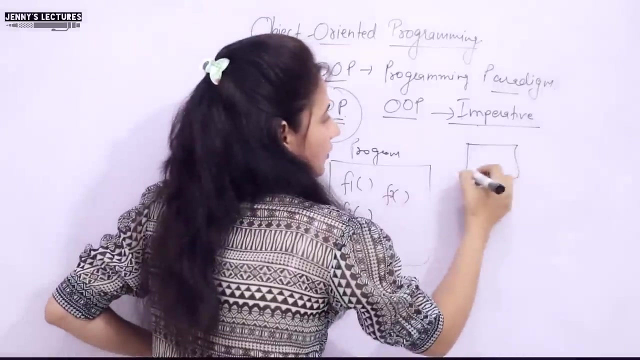 So in this case, C comes under this category, right, C, Fortran, Pascal, these comes under this POP oriented programming. right Now, see, in this case, we first think about the имер: easy things, right Now, you know. OK, Like first I am going to do, tell you what is a procedure unit, right? So basically, 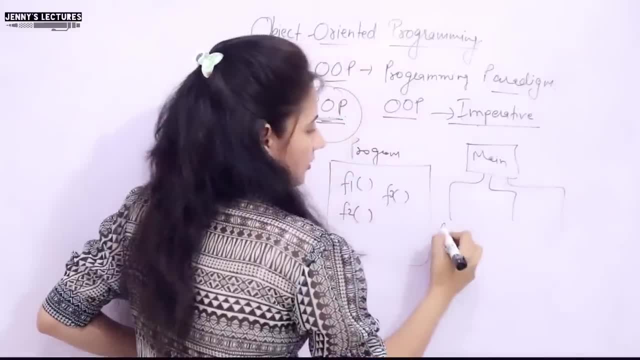 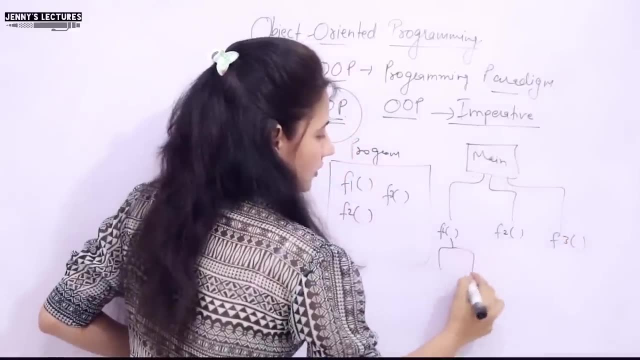 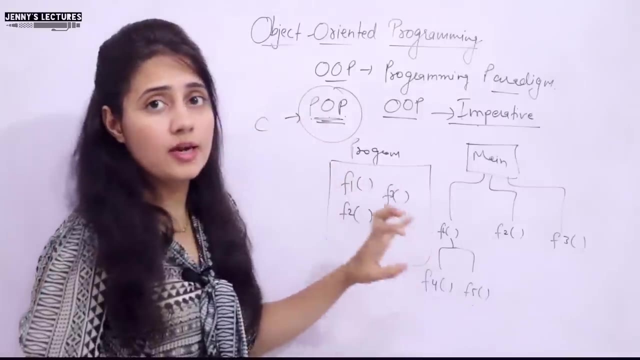 basically C should be the just like a形 function in which we can get some information right simple, we get it OOP, function 2, function 3, and these function can further be divided like function 4, function 5, something like this. So program is divided into parts that are known as procedure or 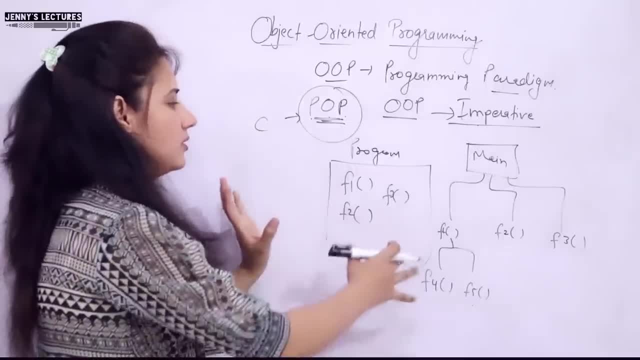 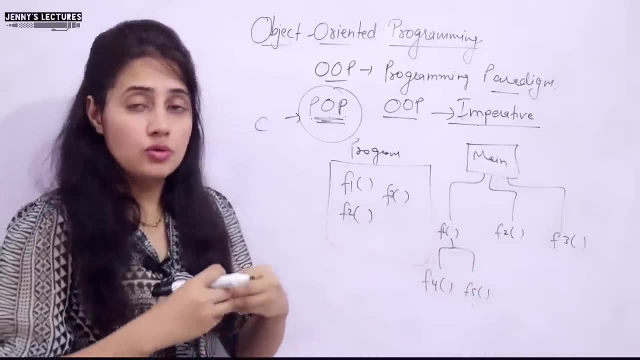 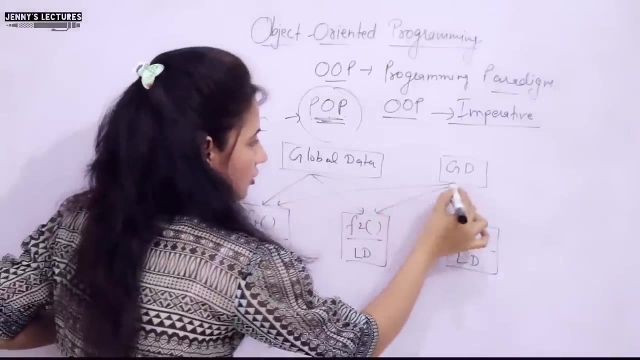 function right Now. these functions are interdependent. you can say: These functions are having their local data, also local data as well as they share global data, something like this We have. so here we have local data as well as global data. These are three functions. 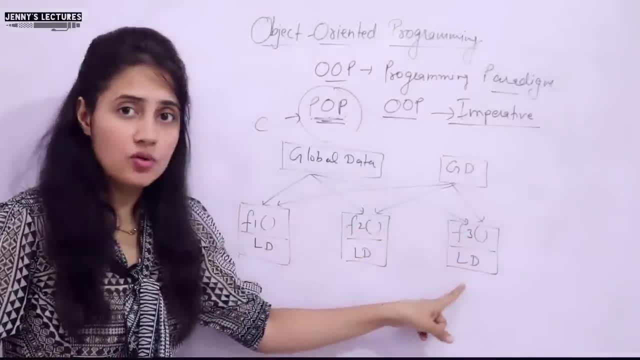 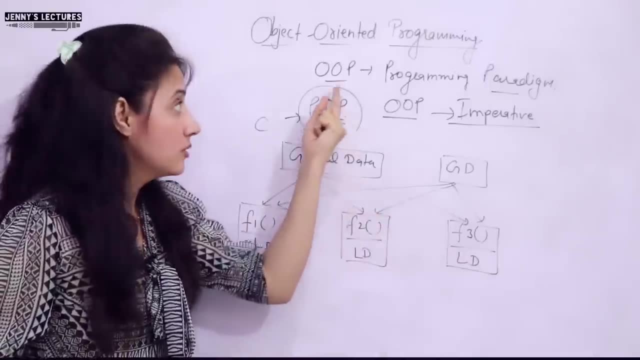 for example, every function is having its own local data- ld means local data and gd means global data- and each and every function can share global data. In this POP programming paradigm, we have global data and more focus is on global data right. Every function share. 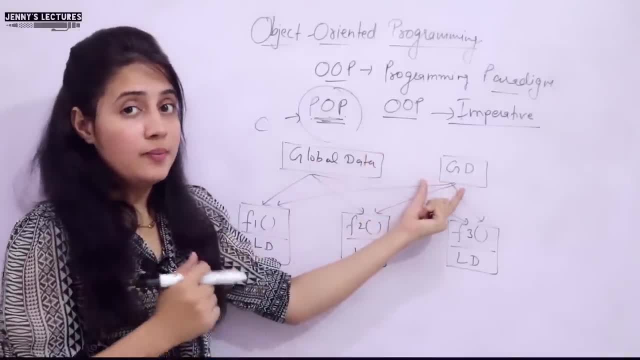 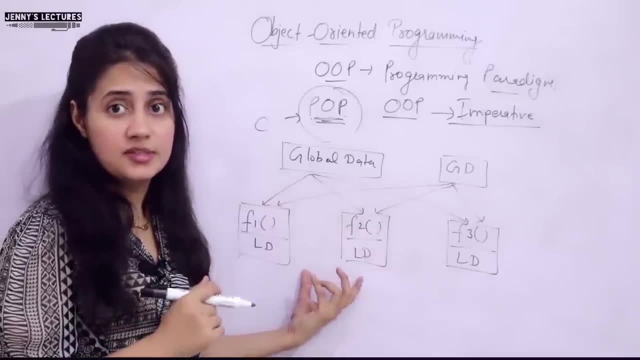 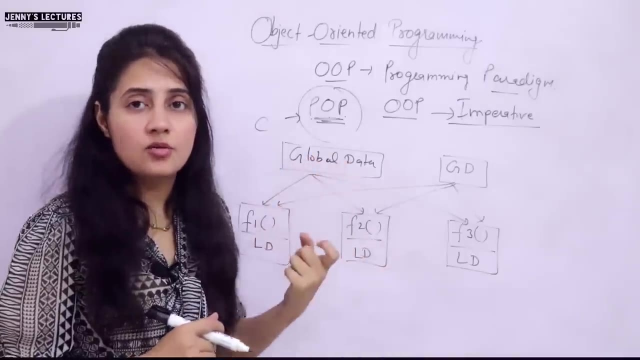 more and more global data. Now the problem here is what? So data movement is more, So data is less secure. in this case, This function can update this data right. Also, this function can also update this data, So data would be less secure- something like this We have. 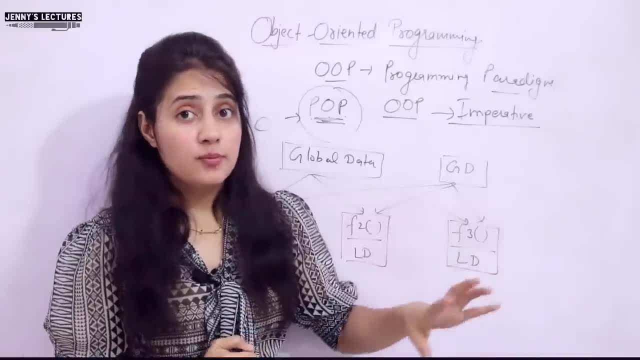 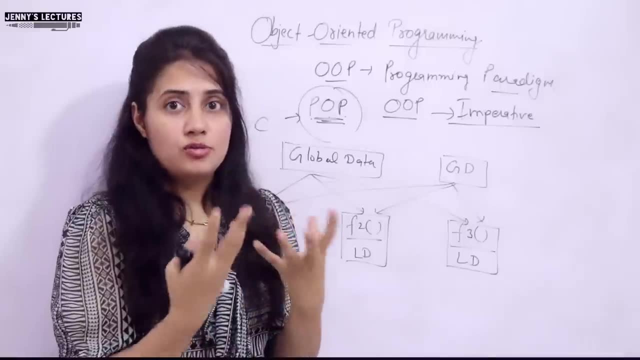 you have kept some money in the locker in your house and suppose each and every person in your house can access that locker. like every person may be- it is your maid or the gardener or your driver- every person in your house. Your house may be considered as a large program. 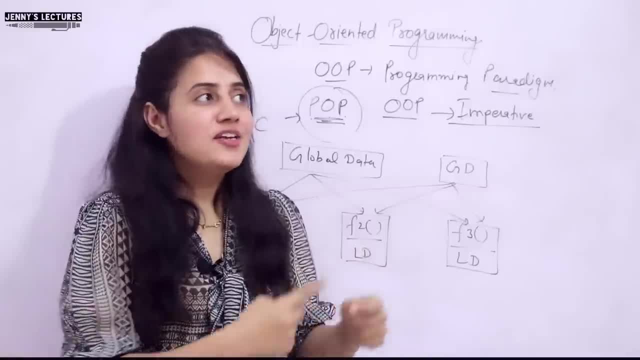 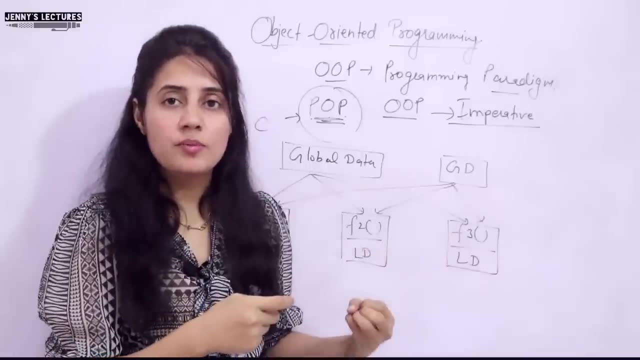 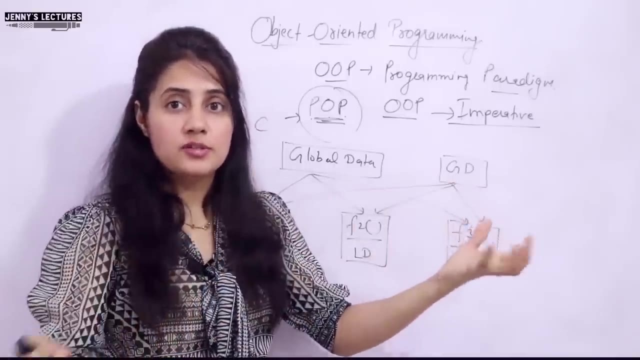 And each and individual is function something like this And each and every can access that locker. So is money safe there? No, Anyone can withdraw money. Anyone can take money from that thing. Suppose I have put 10,000 in there and another person took 5,000.. 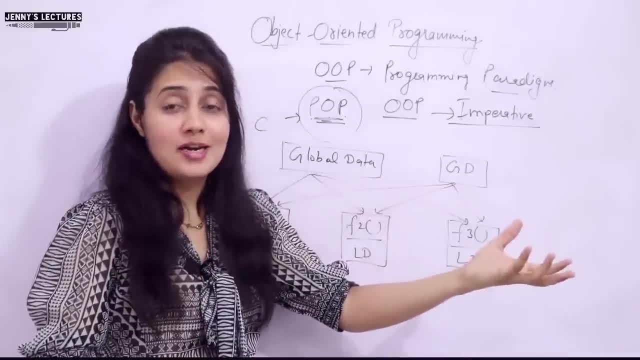 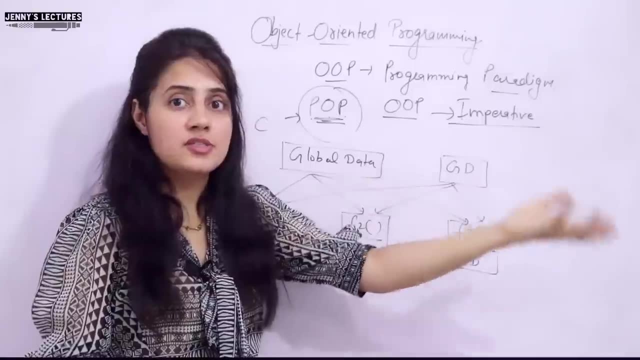 Still, I think that there are 10,000 rupees. Right, But there are now 5,000 rupees only, And suppose I need 8,000.. So I think that there are 10,000 rupees. Let me just take money. 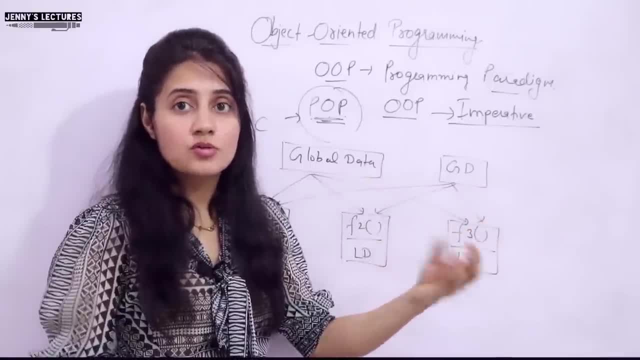 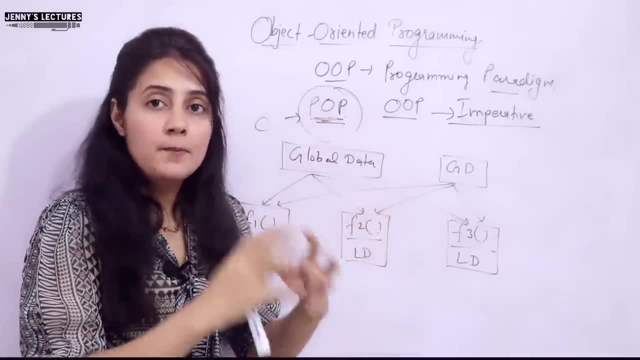 But when I see that there are only 5,000 rupees, So the money is not secure. Same data is not secure in processor oriented programming. This is the main reason you can say Why we switch to object oriented programming, Right. 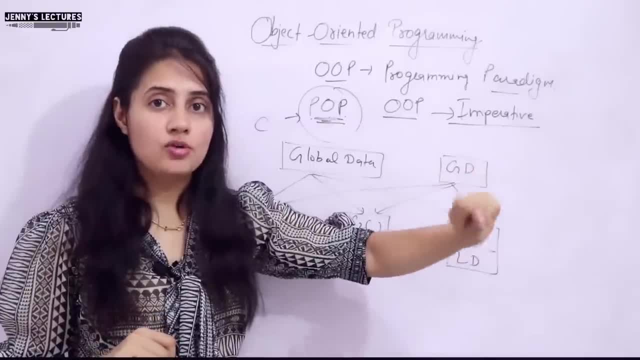 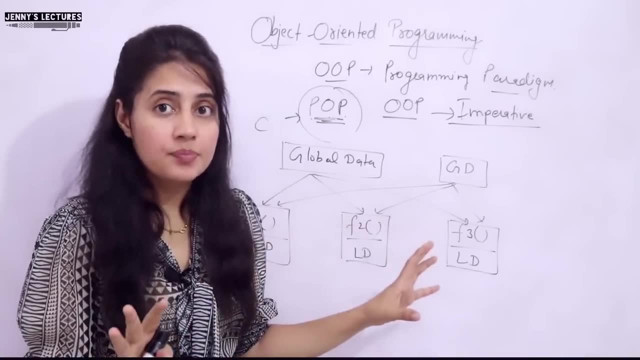 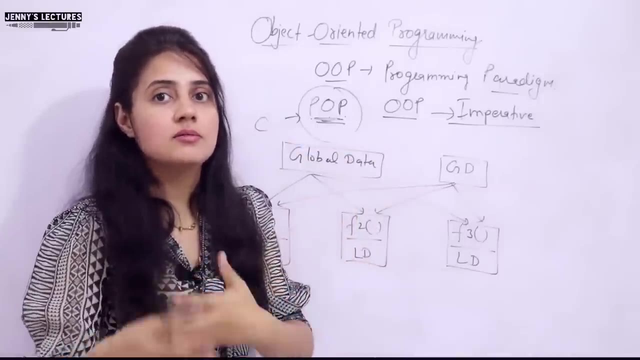 Because the data security, the security of data, is more. in that case, Here we focus on the algorithm- How to do the task- rather than the data. But in object oriented programming We focus on more on the data rather than how to do the task. 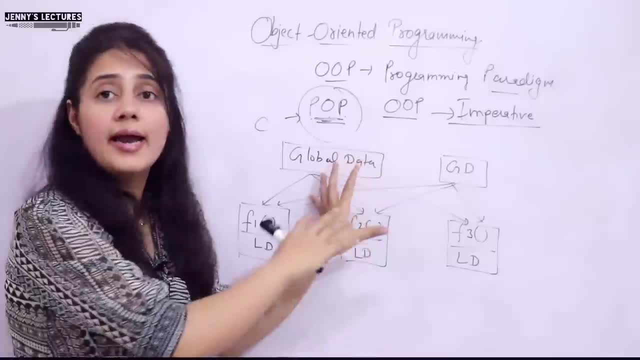 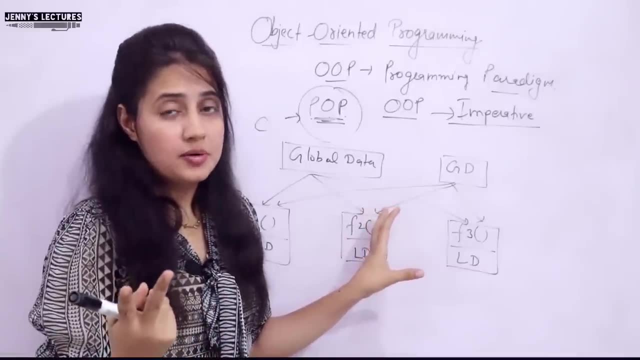 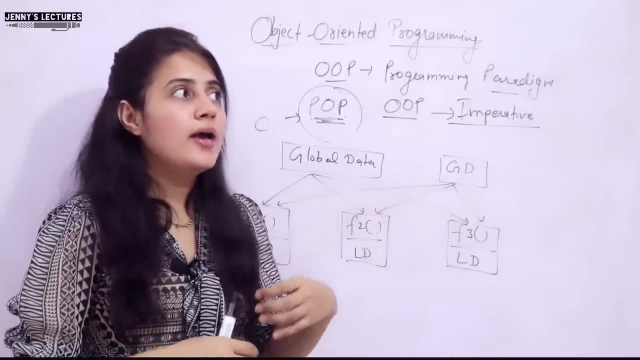 Fine, And in this case also suppose and see scalability. It is not well suited for one thing in which we need more security. Second thing, large and complex scalable applications, The applications which require actively updated and maintenance. This approach is not suitable. 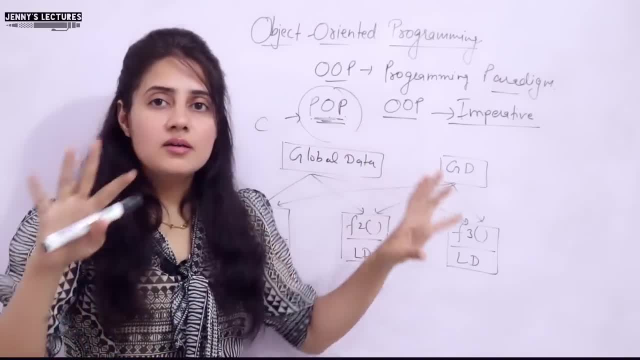 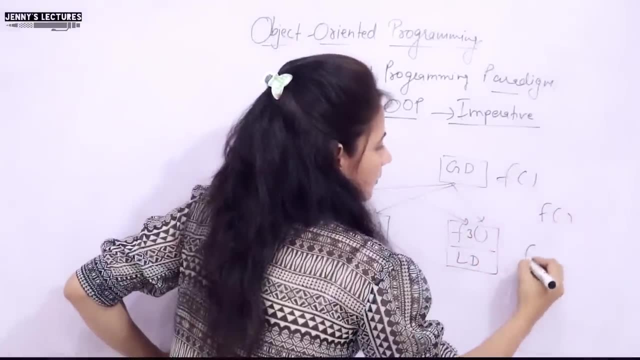 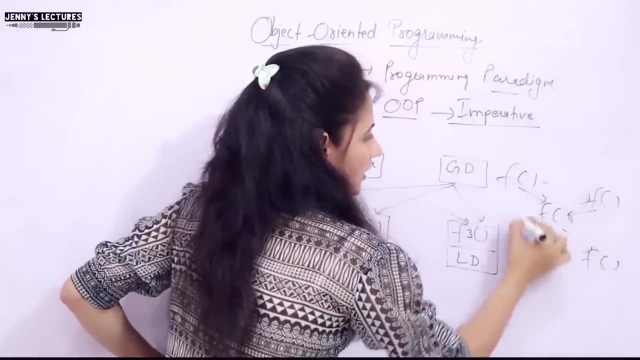 Approach is not suitable for those things Because there are interdependency, more and more interdependency, among these functions. Many functions are there, Right, Many functions are there, calling each and every function something like this. So see the interdependency of the code. 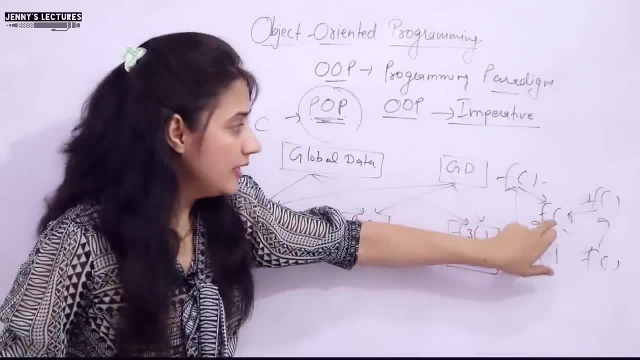 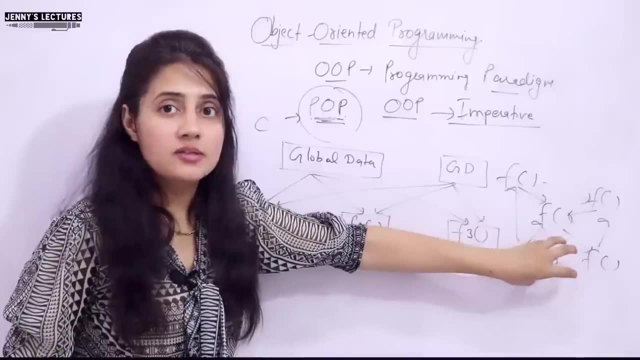 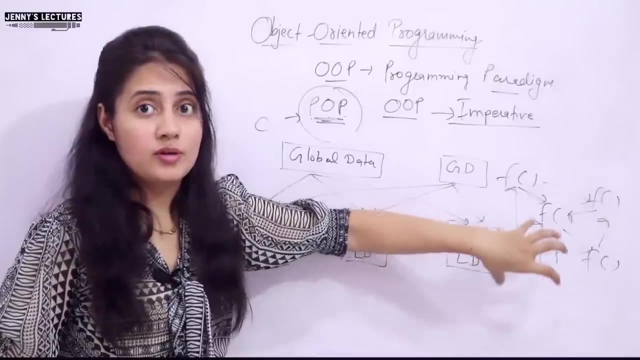 If you update in any one function, this could lead to the updation in any other function also. Right, If you want to add something, some new feature, some new function, that is also very complex because of the interdependency code- spaghetti code. we, you know, call it. 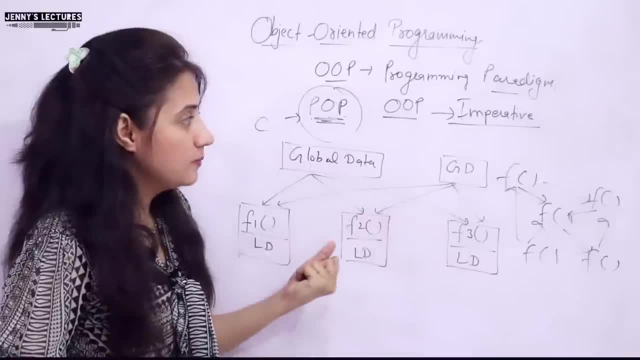 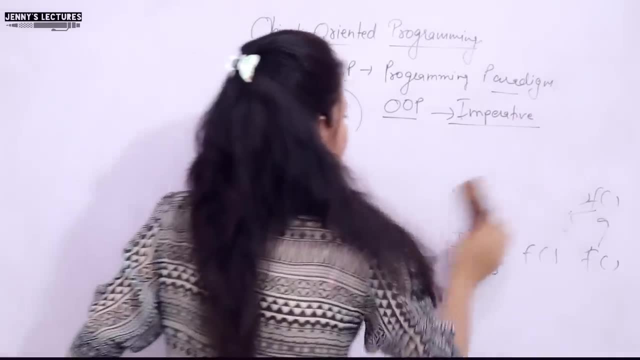 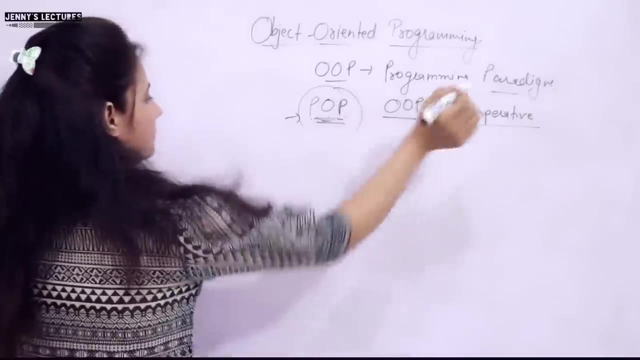 So scalability is also not there, right, Security is not there. Fine, So now why? in OOPS we have security. See general structure of this. object oriented programming is what? In this we do something like: Uh, We have data and we have function. 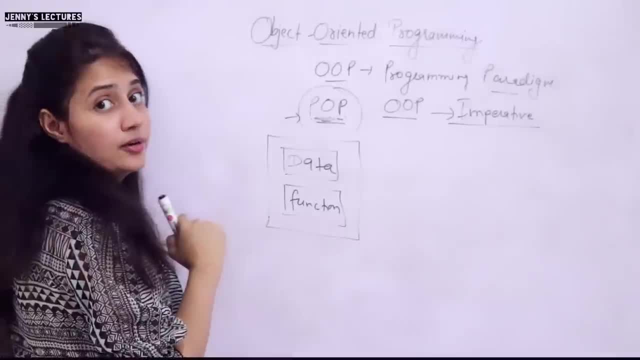 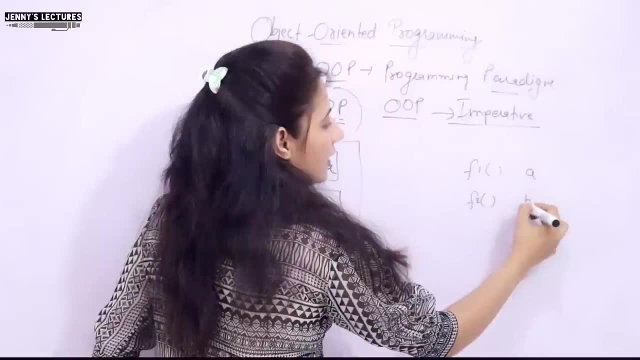 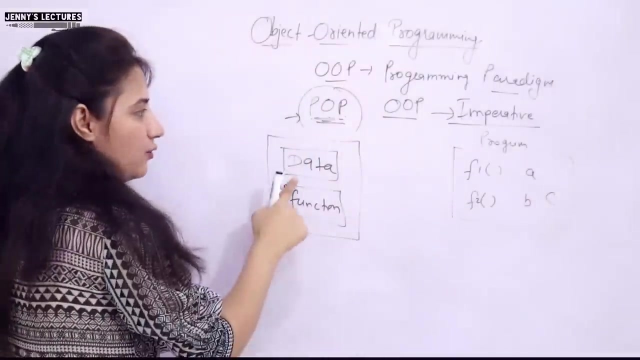 These would be wrapped into a single unit. Then in POP we have function one, suppose function two, and we have our data A, B, C, and this is our program, Something like this. We divide this, But here we do what. 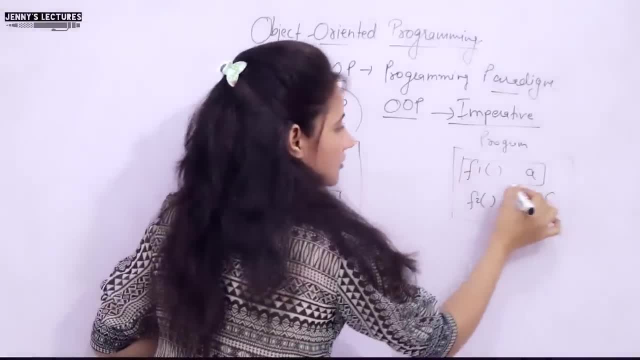 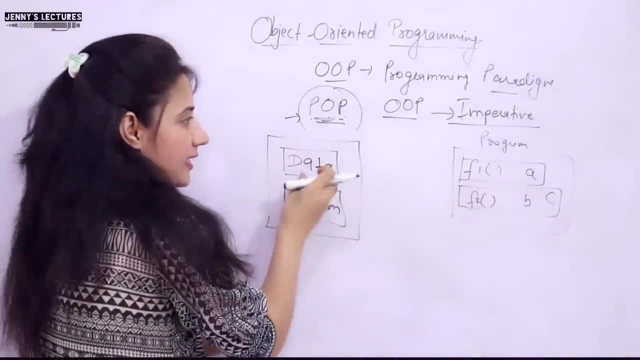 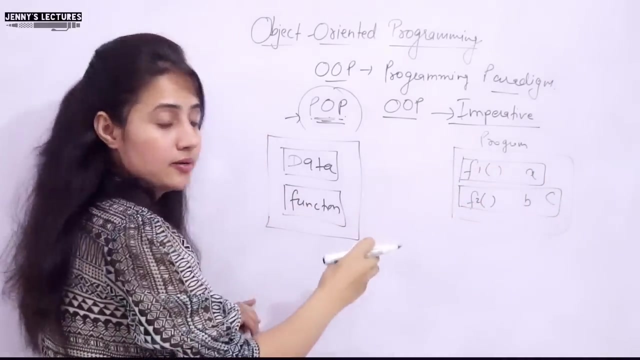 We divide this, We divide this, We separate these things, We separate these things Right, We wrap up these things, The data to the function. So this data would be, you can say, updated by this function only. So less communication would be there. 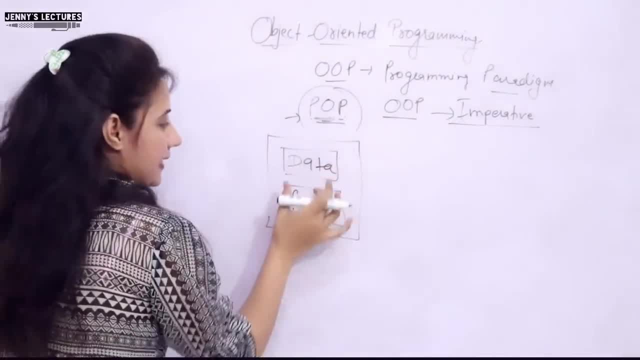 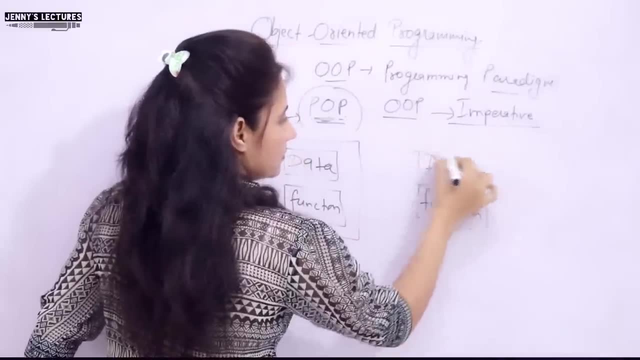 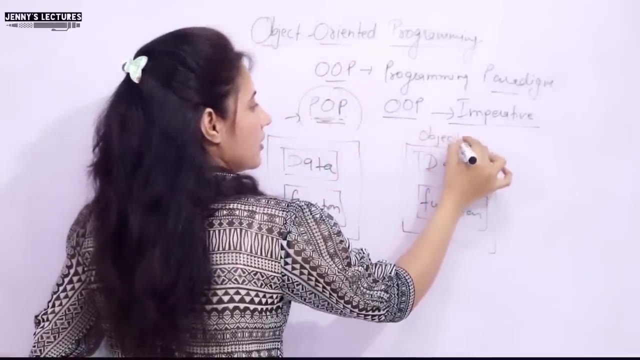 What would be the general? uh no, you can say the structure: data plus function. Here also we have data plus function, something like this, And We wrap up these things And this complete is known as object. This is known as object. 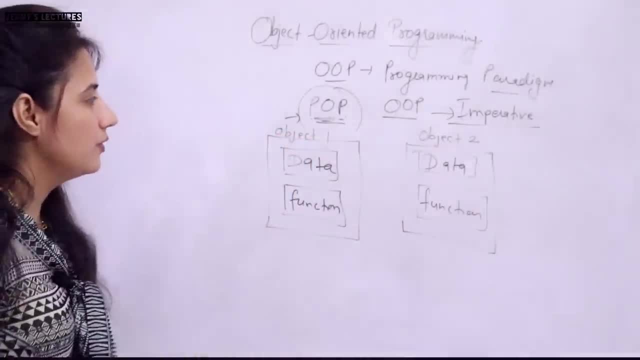 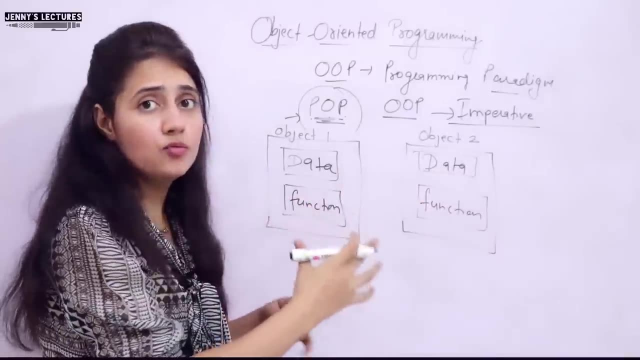 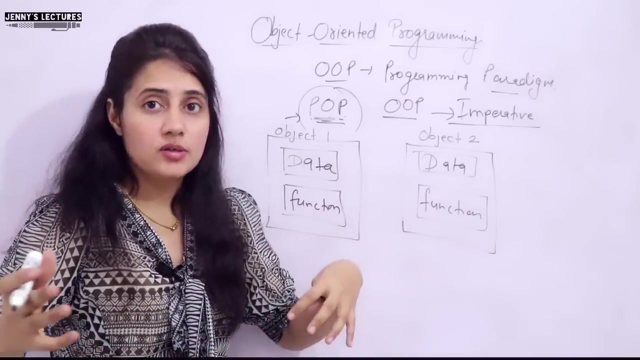 Suppose object one, object two, one more object. is there object three? right, So see, we have wrapped up these things. So the data movement would be less. In POP, data movement was more Freely. data can move from one function to other another function. 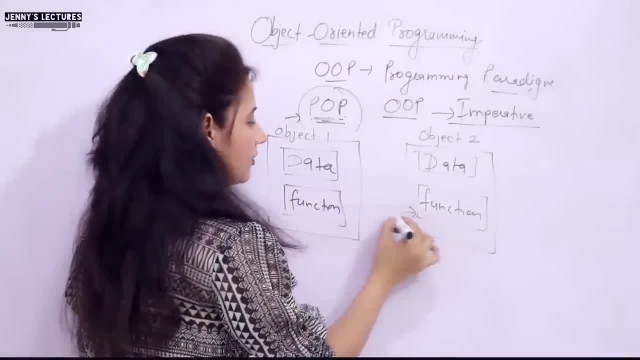 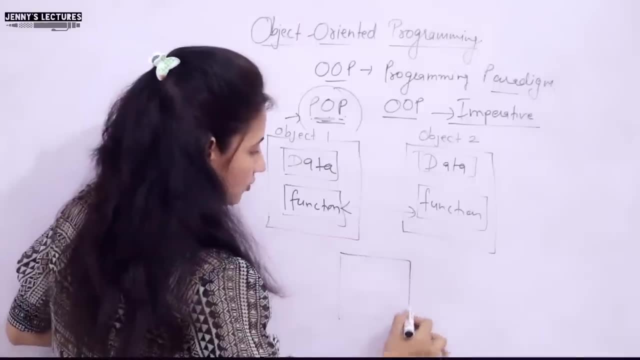 Here, yeah, object can communicate with each other with the help of Message passing. how it could be done that we'll also discuss in later video. Suppose we have another object also here- object three- so they can communicate with message passing. 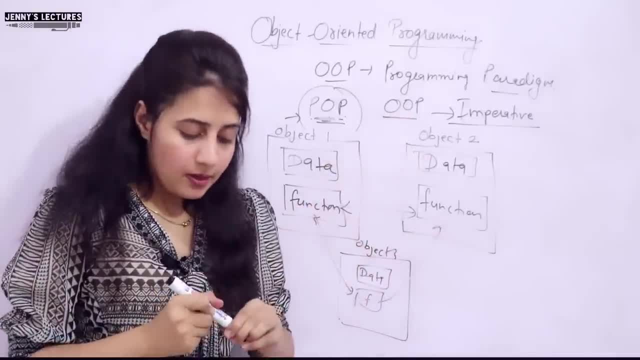 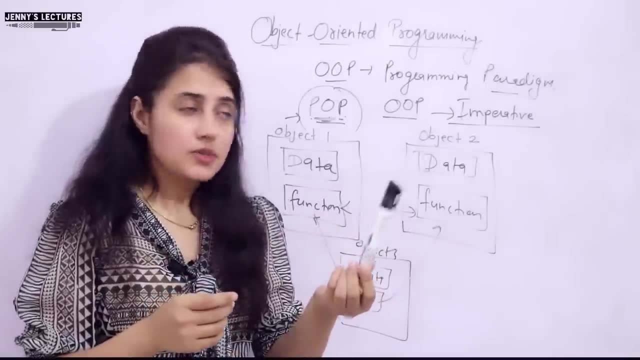 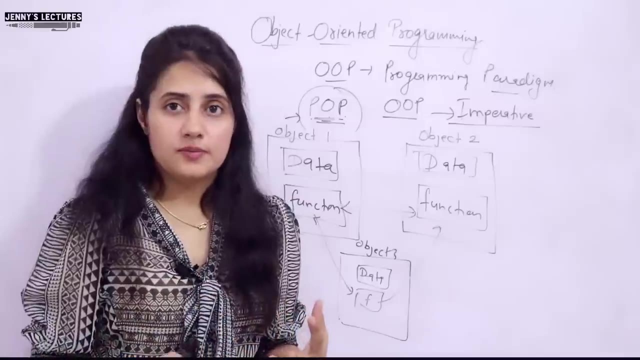 So in object. now, what is this object? See, object is, you can say, a real world entity, something like this: This marker is an object. this whiteboard duster camera, my bottle table bed, These are objects, right? 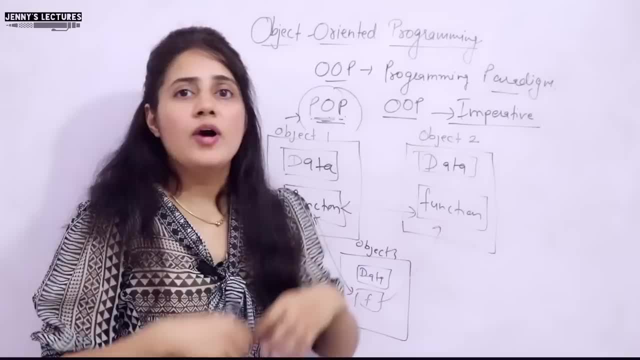 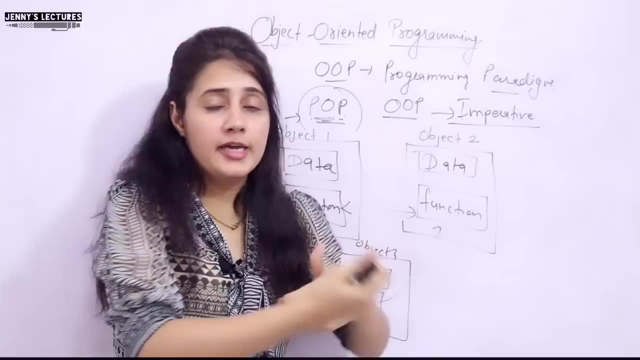 We are also objects like suppose we want to, why we do programming? because we? it's not like that. We just want to write the simple, simple program, just to add two numbers. print Hello world check number is even or odd. reverse a string. 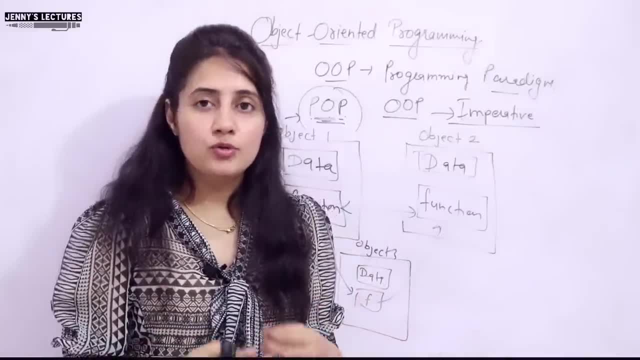 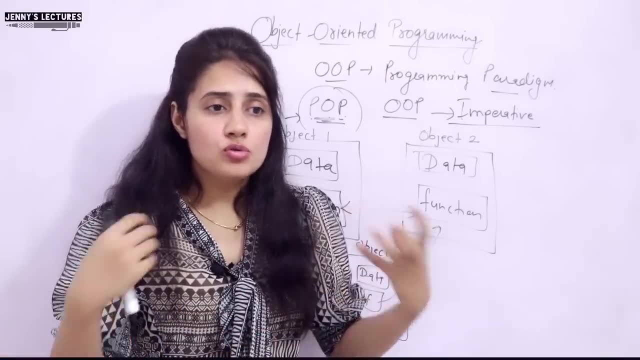 No, these are basics We are. you know, we used to get us familiar with the programming concepts with these basic programs. Ultimately, what we want to do? obviously, we want to solve some tasks, some problems related to real world, like we are. 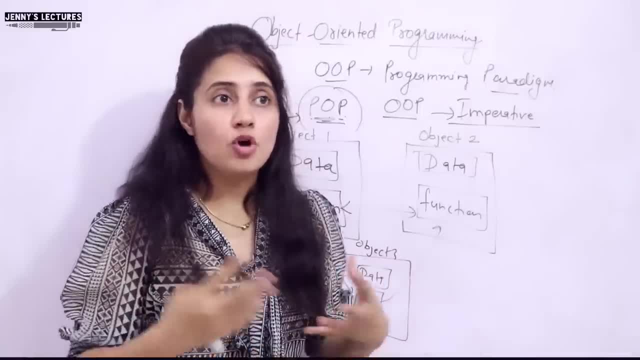 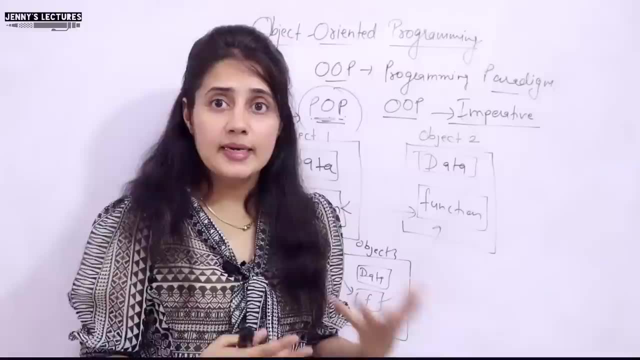 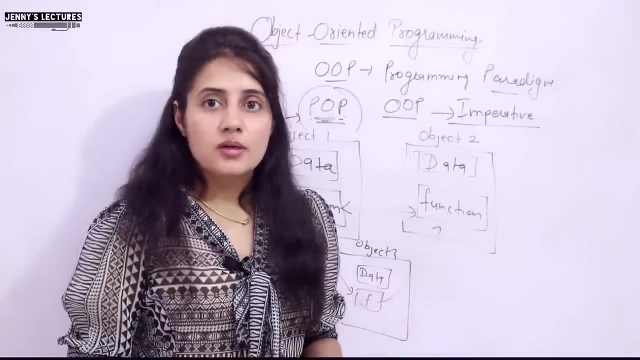 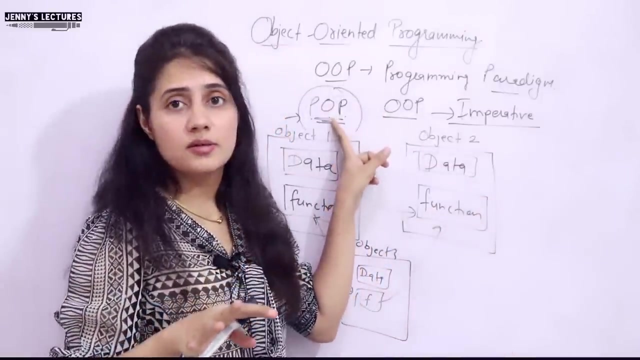 Creating software: hospital management system, library management system, shopping cart. some e-commerce websites are there- Amazon, Flipkart- So they are being created. Behind that there is a complex code in any programming language And to create, to solve these kind of problems, processor oriented programming. this is not suitable for the complex and large scale applications. 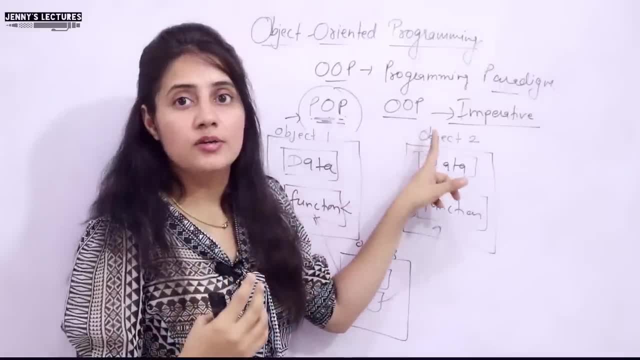 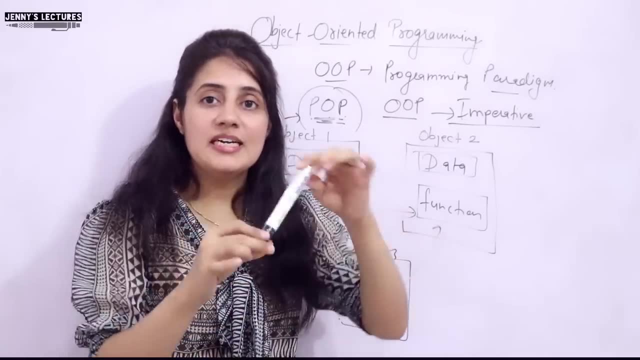 Because the main reason is: what is the data security? So that's why we move to object oriented programming. Now, object is what real world entity? a real world entity? We, can you know, represent this real world entity in the form of programming. 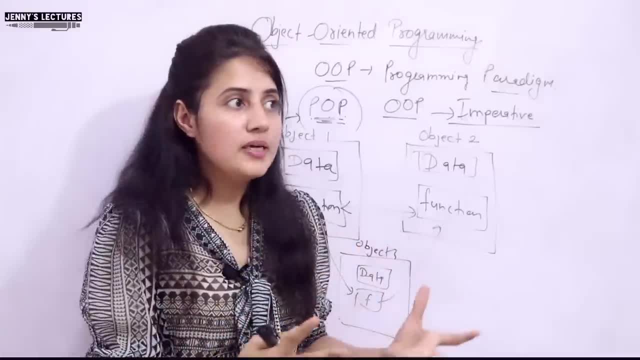 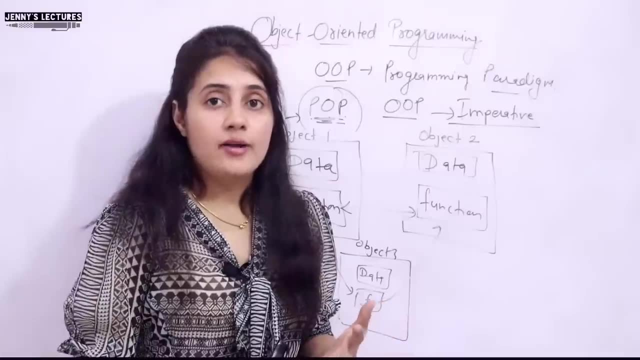 And this is known as object right, Like for a shopping cart, that website, customer. object: shopping cart is a customer, sorry, an object. and what objects can be there like a product? So in short, we can say objects, you know. 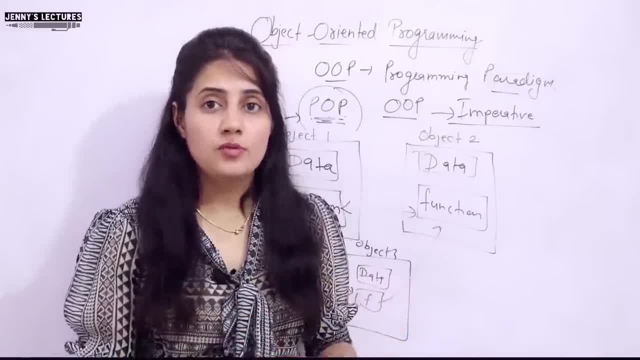 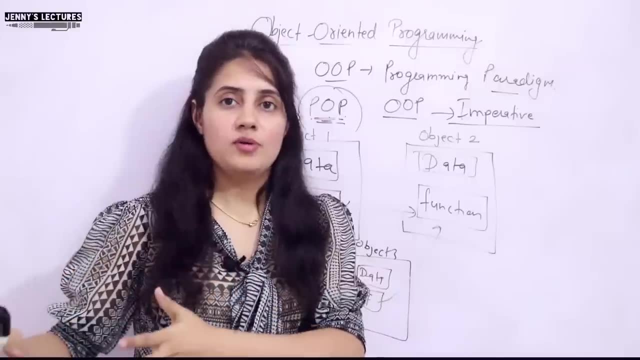 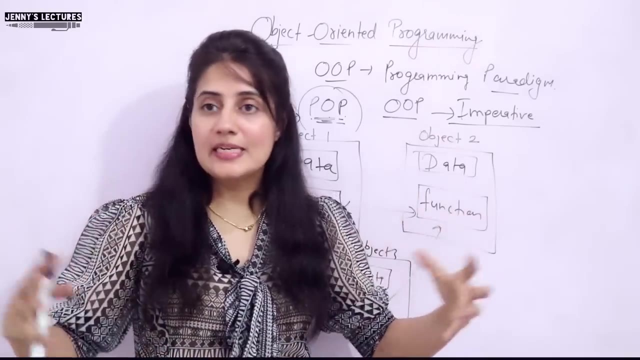 corresponds to the things which found in real world right, So it is close to the real world problems, right To solve real world problems, to represent the data which is actually present in the real world, we use this concept: object oriented programming. 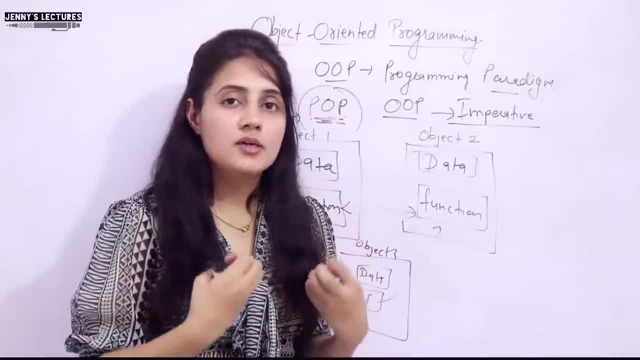 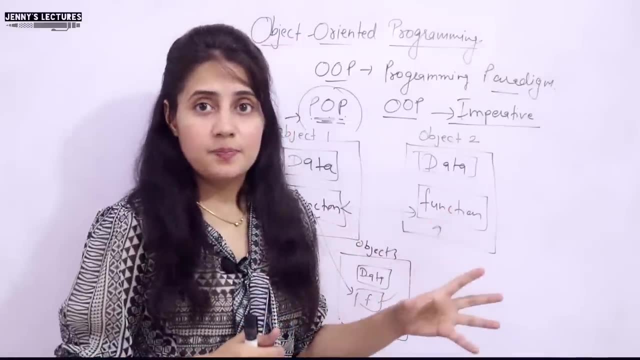 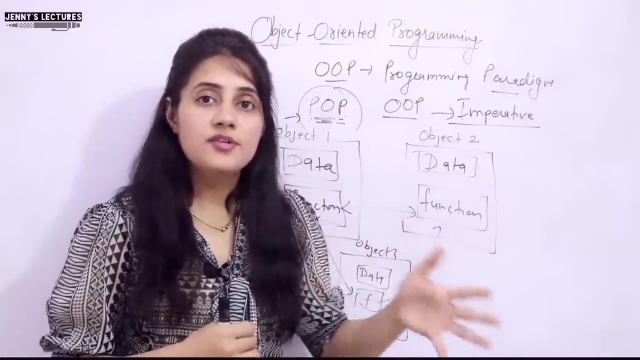 And each object is having its own data. Or you can say the state and behavior, attribute behavior. See suppose employer is a class, so object can be Ram Shyam Jenny. these are different, different objects of that class. 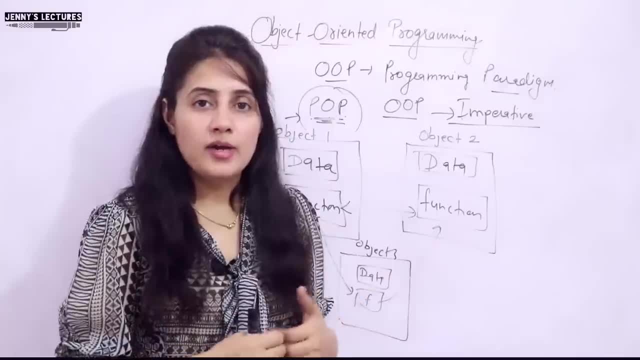 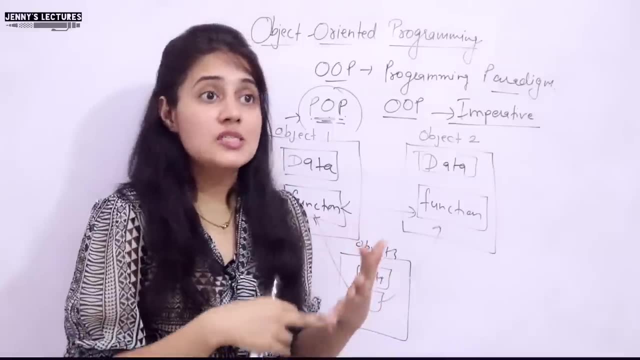 So every object is having its own attribute, like height, color, weight, right, And these are the- you can say- attributes, or the data or the state of the object right Which we represent in the form of variables. And another thing is behavior. 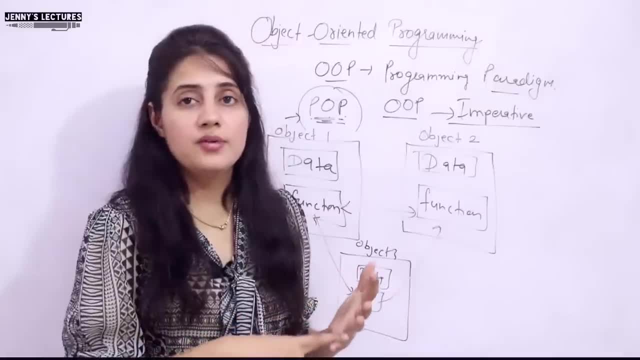 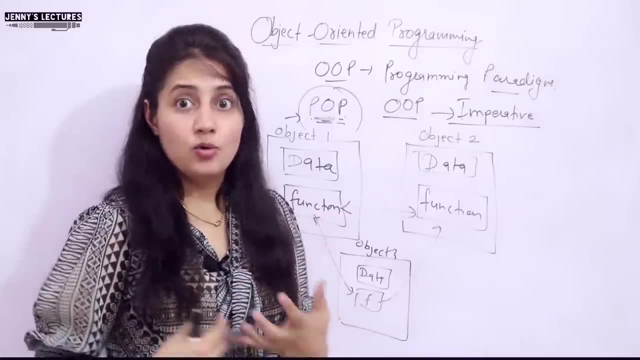 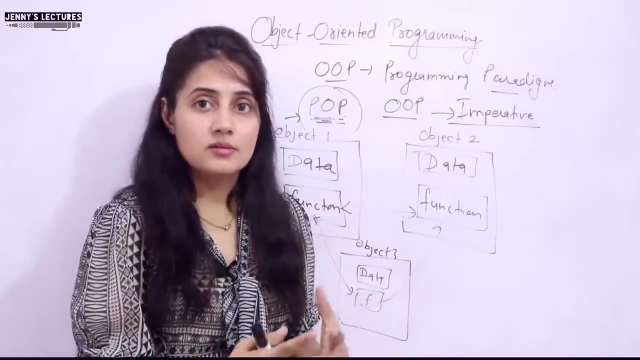 Behavior of the object. Behavior can be like behavior, like I can code, I can sleep. can sleep can eat can code. So these are. we represent the behavior in the form of functions method in a class. right Class is just a blueprint. 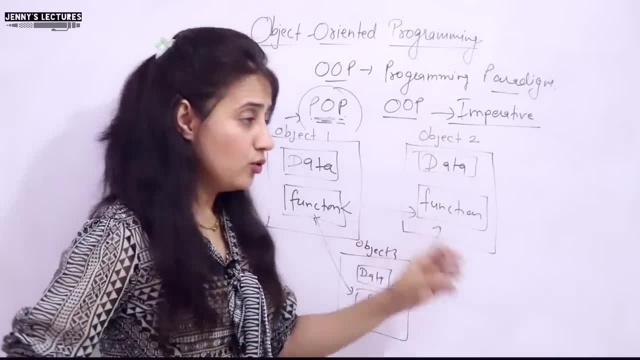 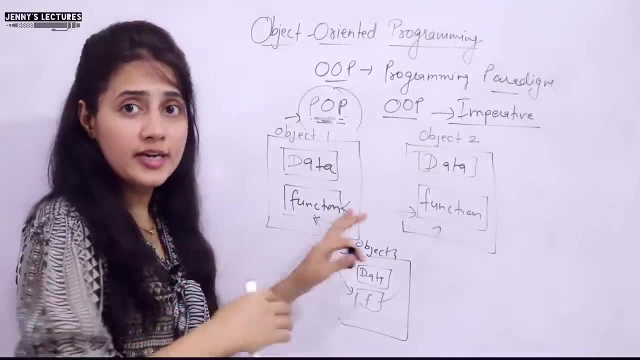 In detail. we'll discuss what is class and object and everything. The main motto of this video is just to get you familiar with object oriented programming, how it is different from POP, So how data sets, Data security comes here. Another feature is what data security? 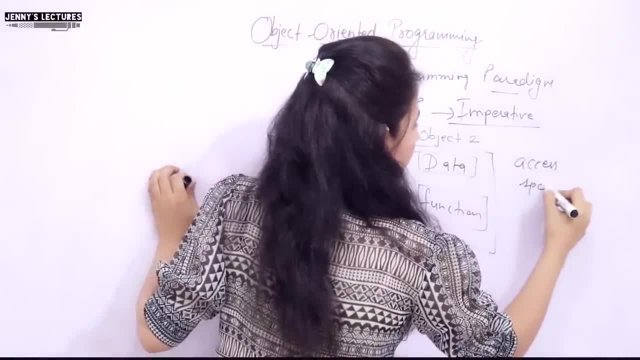 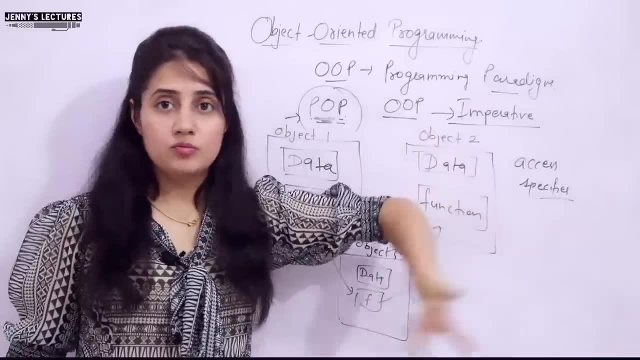 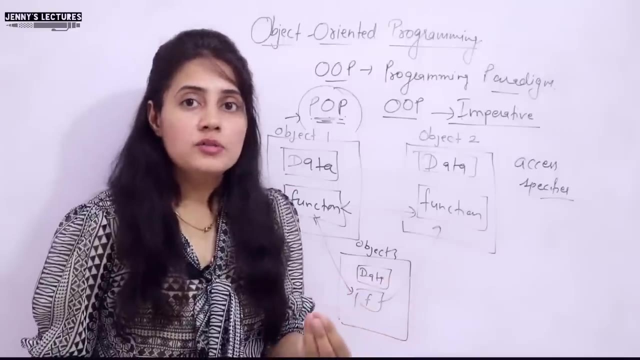 Here we have access specifiers Means private, public, protected. If you want that the data any nobody can access that data, you can keep that data private. So your data is secure. If you want that only few person can access that data, you can keep it protected. 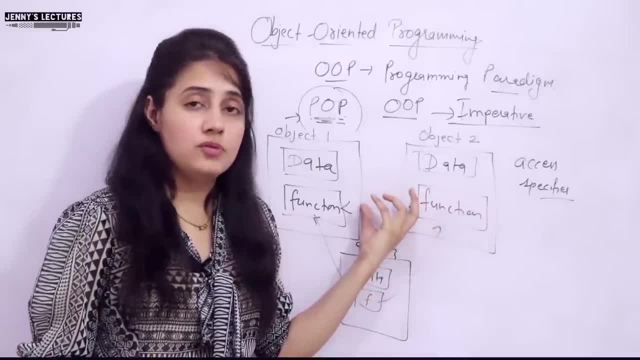 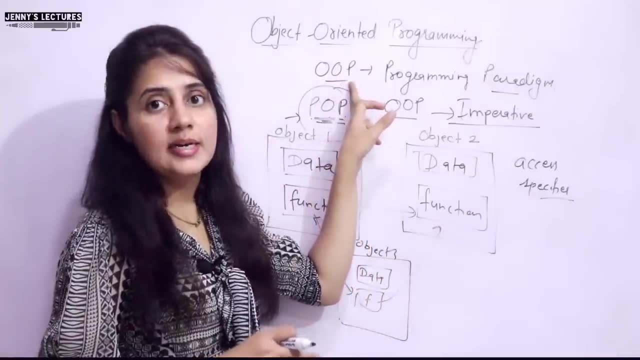 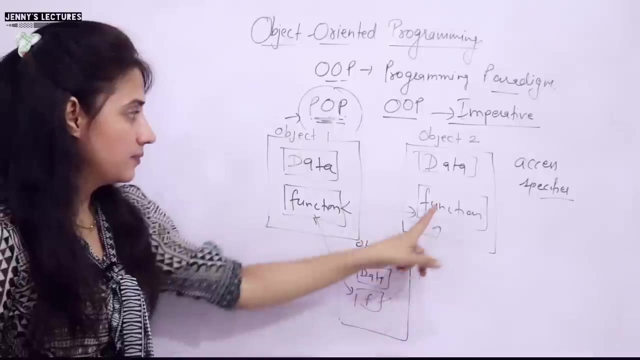 If you want that some data is, it's no harm if anybody can access that data so you can keep that data public. So we have access specifier concept in OOP. That is why data is secure. One thing in this case you can say: the program is divided into parts which are known as objects. 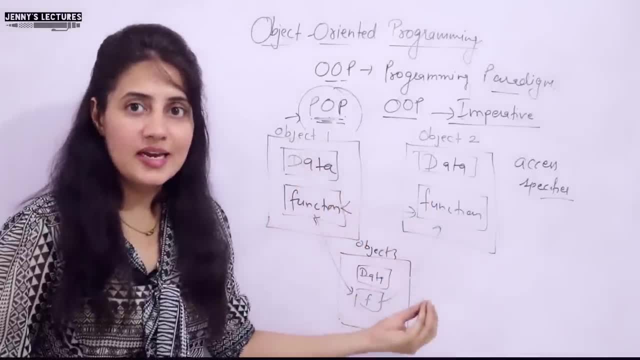 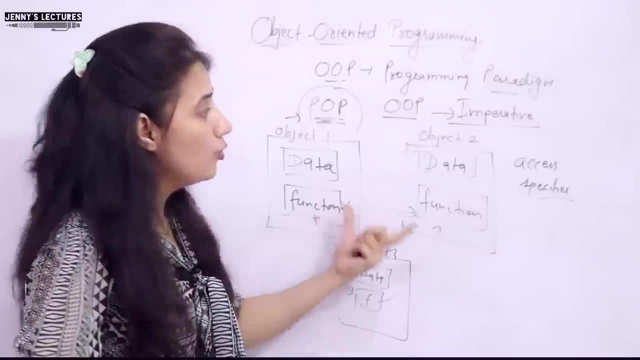 And each object is having its own attributes. or you can say: state and behavior right And object can communicate through message passing right, And here the code. reusability is also there because of inheritance. One concept, OOP's concept, is inheritance.